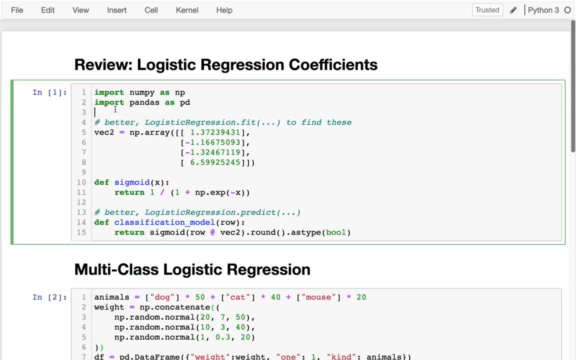 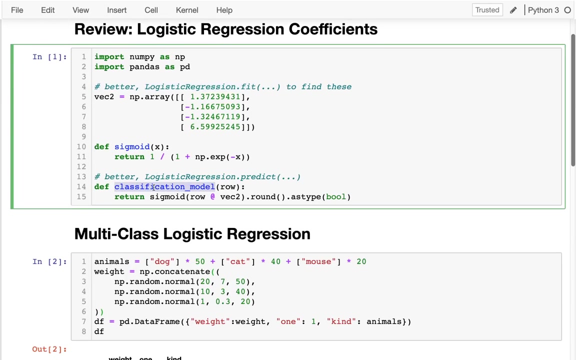 of data and say: well, oh, either true or false. That problem is called binary classification, and it would be based on something very similar to what we would use for layer regression. We would have a bunch of coefficients, probably ones that we found with logistic regressionfet, and then we would have our classification model, which would return. 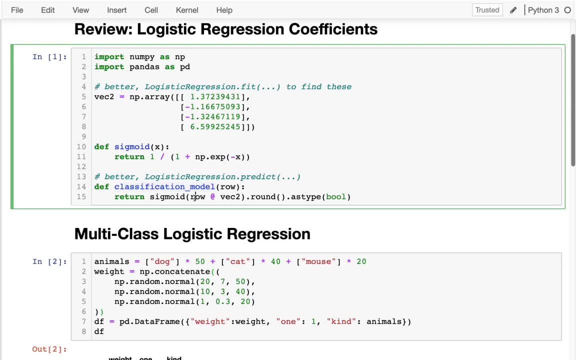 either true or false. So the way we would do that is we would take a row of data and multiply it by our coefficients to get a number. Then we would take the sigmoid of that number to convert it to something between zero and one. We would round it to get exactly zero or one. 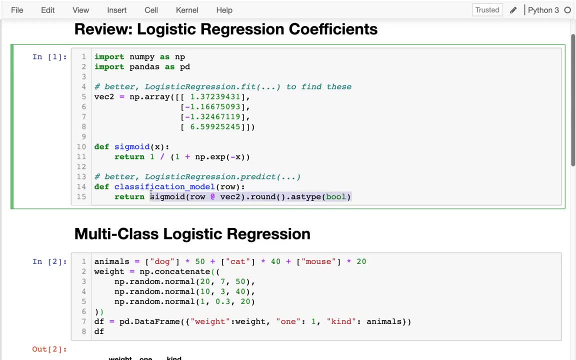 Then we would treat a one as a true and zero as a false. So that's what we would do. and then, of course, rather than actually kind of dealing with the coefficients directly this way, we would probably just kind of use this handy logistic regression dot predict. Okay, that's great, right. 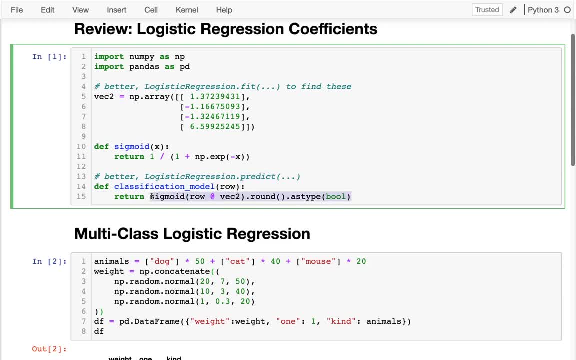 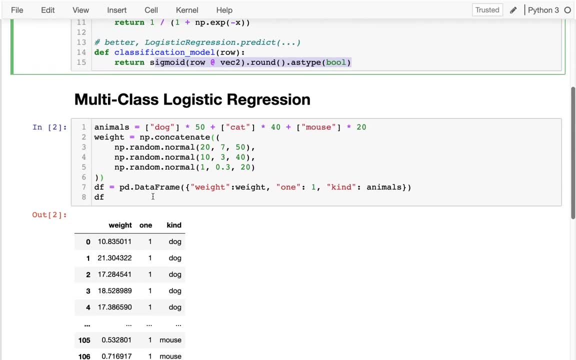 we can take these numbers and basically get a true or false, But what are we going to do if we want to have more than two categories? For example, down here I produced a data set where I have a bunch of animals and we had no other way to do that. So what we're going to do is we're going to take 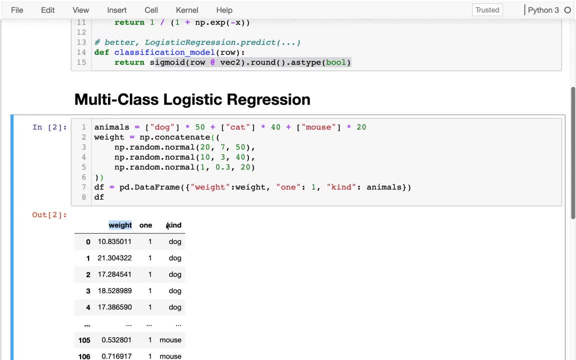 these numbers and basically get a true or false. What are we going to do if we want to have more than two categories? For example, down here I produced a data set where I have a bunch of animals and we know the weight of those animals in pounds and then we know what kind of animal it was. 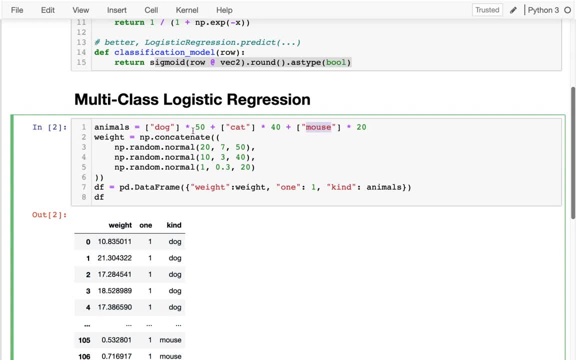 and we can have either dogs or mice, and then, of course, those are probably from heaviest to lightest. I just made up the data for that, and so how can we do that right? This is just returning a true or a false right. when I convert to a 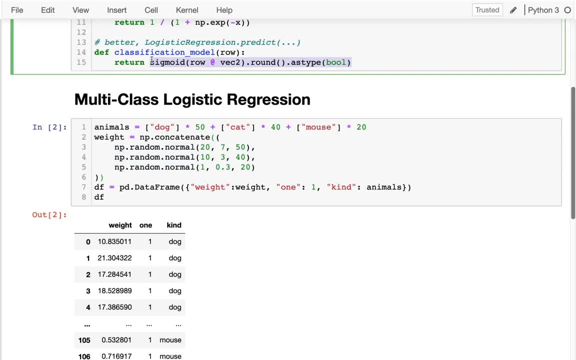 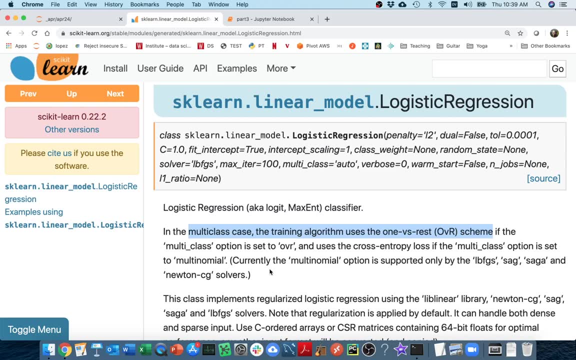 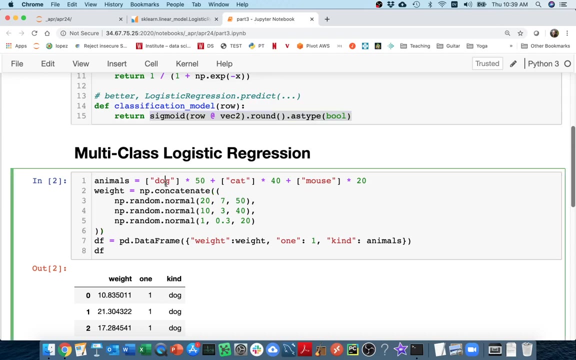 boolean, but how could I convert that to, you know, a dog, cat or mouse? And it turns out that what logistic regression is doing is something called OVR- one versus rest, and what it's realizing is that, well, we have three different things, and so it's actually going to train three logistic regressions each of. 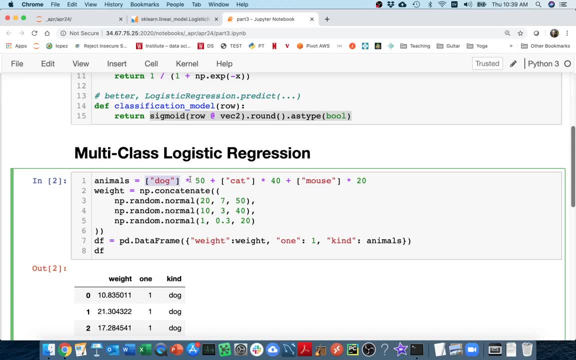 which gives a true or false right. So there's going to be one that says true or false. is it a dog True or false? is it a cat True or false, is it a mouse? So I'm actually going to have three logistic regressions and the key that we're going to try to. 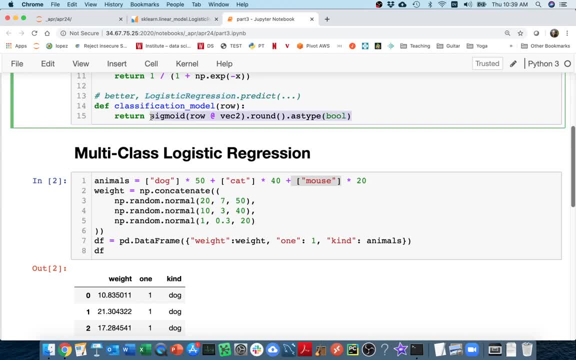 deal with is, instead of each of these three logistic regressions being true or false, we're just going to take this part of it and that will tell us whether, well, how confident the logistic regression is, that it's a dog, how confident is the cat? 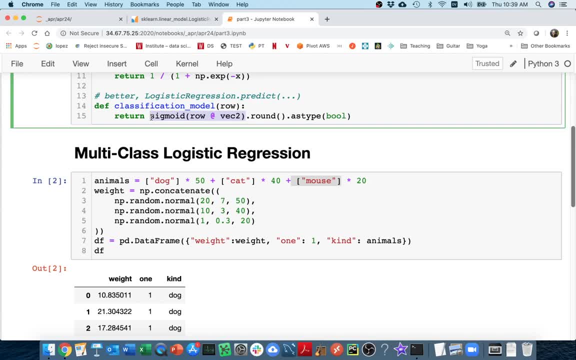 logistic regression that it is, that it's a cat, and then we'll basically see, well, whoever is most confident- is the dog regression most confident, or the cat regression, or the mouse regression? and then we'll kind of go with whatever class is the highest, And logistic regression in Python is automatically doing that. 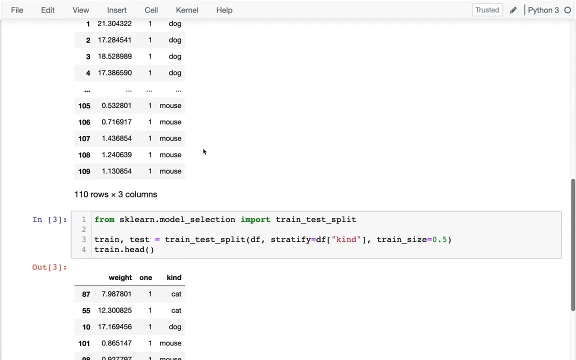 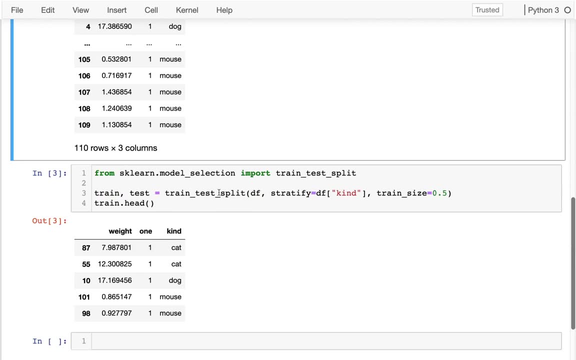 for us. So we're going to kind of peek into that. So here I have my data and you can see I have this ones column that I'm just going to use for kind of illustration purposes later. I'm splitting half and half, stratifying. 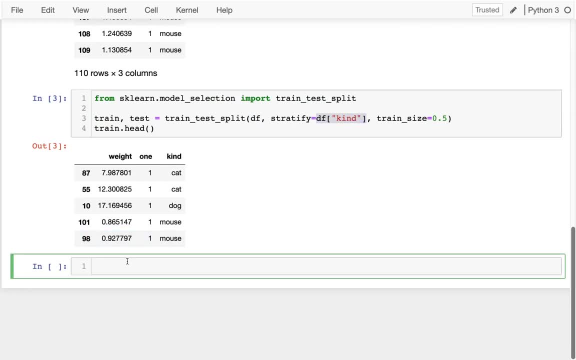 on the kind of animal we have. and let's do a logistic regression on this. I'm going to say from sklearnlinearmodels import logistic regression and I'm going to create one of these And I'm going to hit it. and what do I want to fit it to? Well, I want to fit between my X. 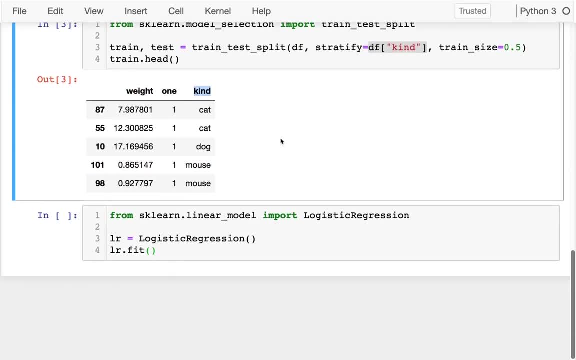 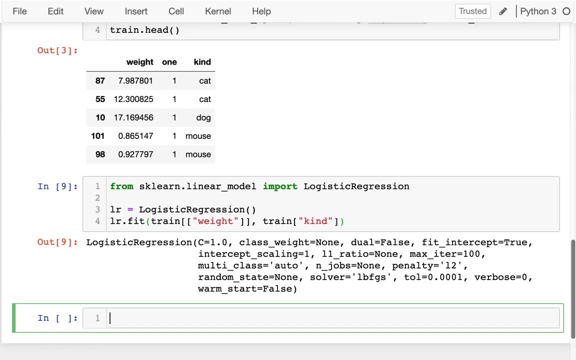 values, the weight and my Y values, the kind I will do that I'm going to say training data and the column I want is weight And then what I'm trying to predict is the kind. So I run that and now I can actually do predictions with it. I actually want to feel like I'm 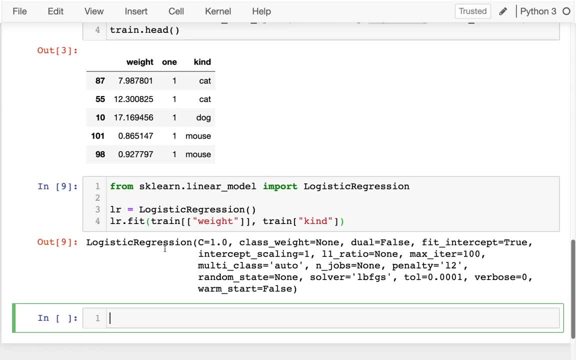 this, And so maybe what I'll do is I will say lrpredict, and what I want to predict is: well, I'm having my training data, I'm going to have my testing data, I'm going to have my test data, like that, and I'm just going to add this as a column to that. 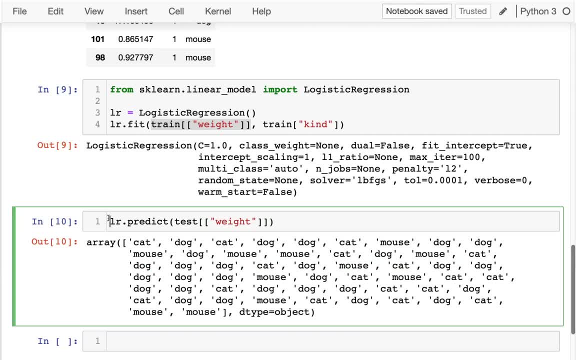 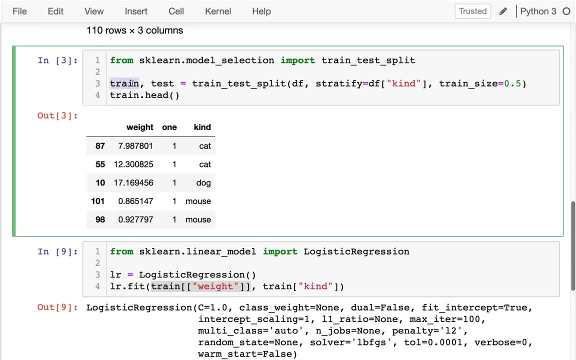 predict table right. So I'm going to say: test data predict equals this. And this right now is going to be a little bit unhappy because I can't add a column to a data frame that is a slice of another data frame, And so to actually do this, I actually have to try to decouple that. So I'm 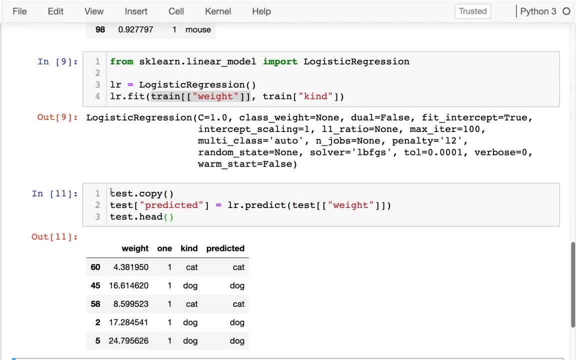 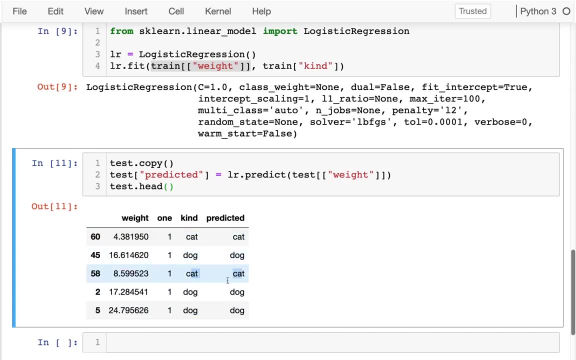 going to do that and take a peek at that, And I can see it's doing pretty well. I mean, you know, there's some cats that are bigger than some dogs, but in general this is going to help me predict it fairly well. But let's actually look at the coefficients and try to see how. 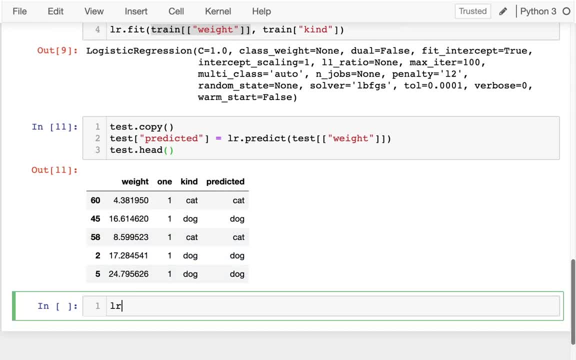 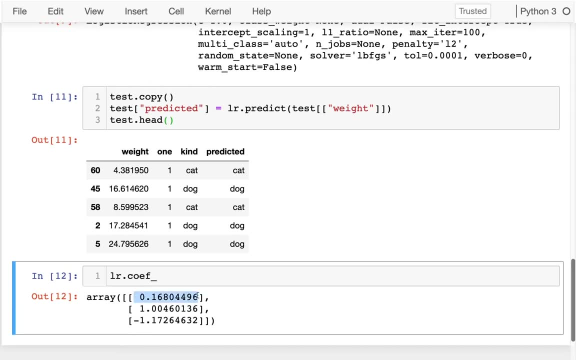 I was making these decisions. I'm going to look at the coefficients, And what you should notice here that's kind of strange is that I have three numbers, right, Three numbers for the coefficients, And actually, if I look at the intercept too, I'm also going to have three numbers there. So 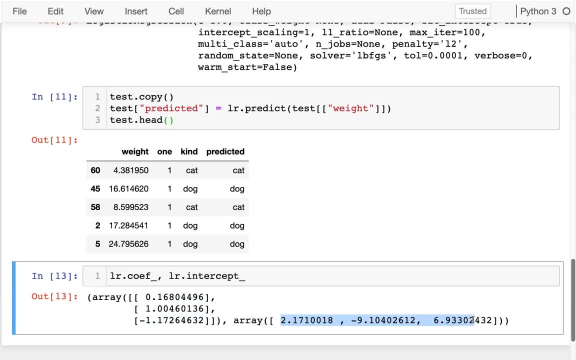 these are the coefficients. This is the intercept. It's kind of weird, right, Because normally, if I'm doing a logistic regression or linear regression, well, I have one value per how many variables I have. I only have one variable, So you might expect that I would just have one coefficient and one intercept. 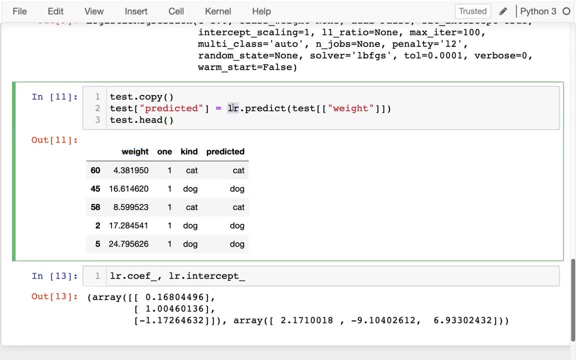 but I have these three And that's because this linear regression- I'm sorry, this logistic regression- actually did it for cats, it did it for dogs and it did it for mice. Okay, So how is it actually making these predictions? And since it has these three, well, let me show you what it's. 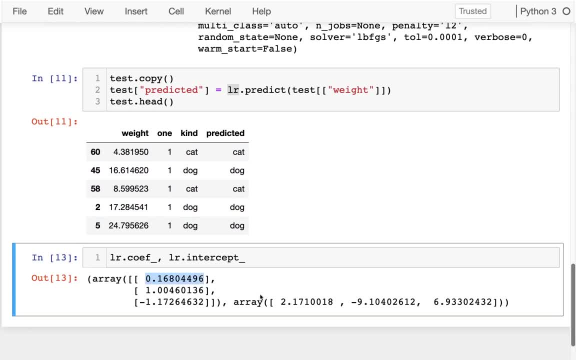 doing. I have to if I want to do the linear algebra behind this. I have to shape this up a little bit. I have to get the coefficients for dog, cat and mouse, each in their own columns. I'm going to have three columns And in the first column I'm going to have the dog coefficients. 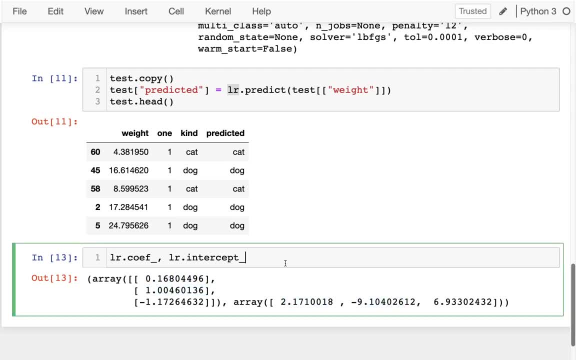 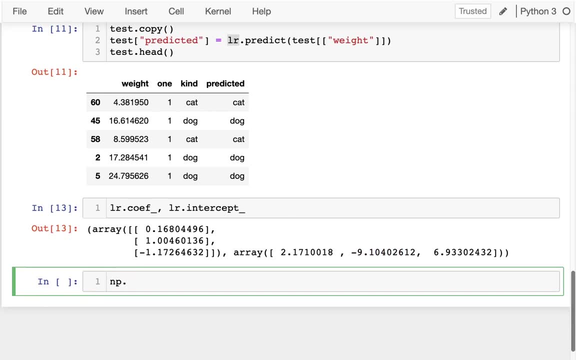 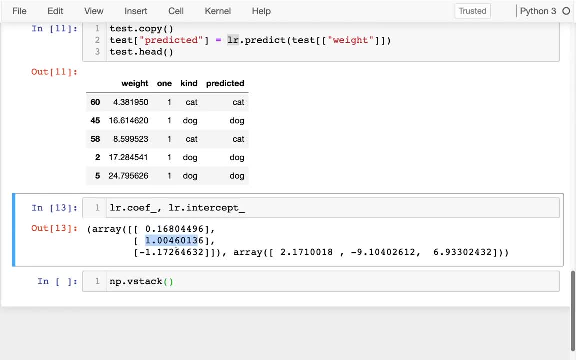 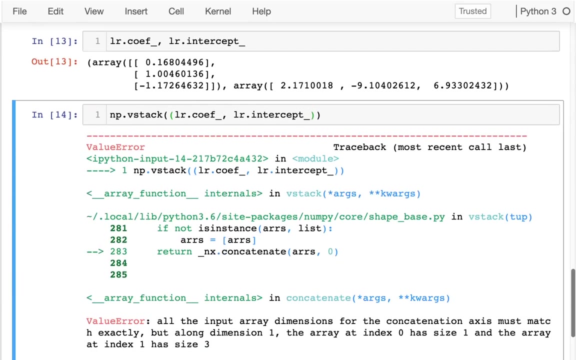 where I can put the coefficients on the variable over these other ones, And so I'm going to do a vertical stack. I have to pass in a tuple of things I can say coefficient and LR, dot intercept, And it's making me unhappy about the shape of it because this one is vertically oriented. 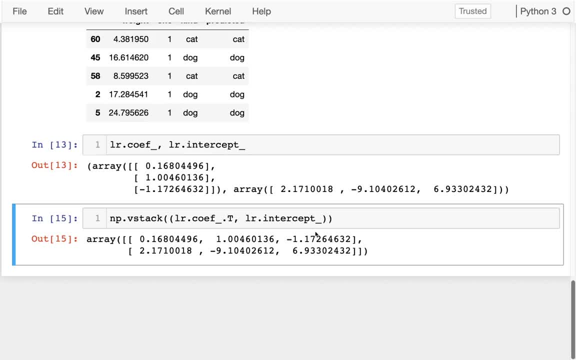 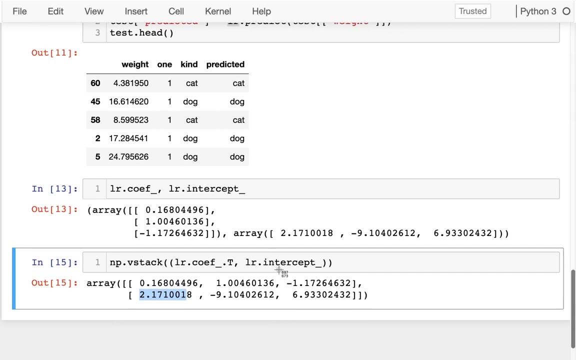 and it needs to be. it needs to be horizontal, like that. Okay, So you can see that I have these numbers here, right? that's? I actually don't know which column it is right. I'm not guaranteed that it's dog first. I could imagine that each of these columns represents the logistic. 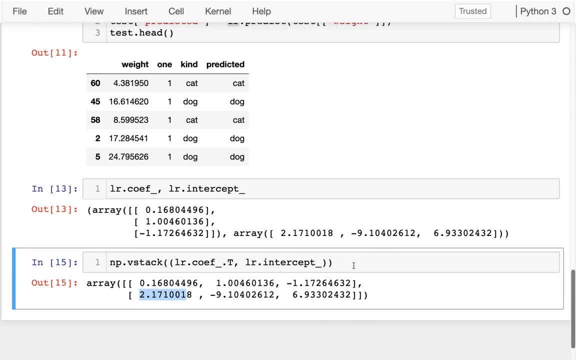 regression coefficients for one of these classes that I have, right? so I'm going to put this in something called coefficients, like. so let me peek at that, and I'm actually going to use these now to multiply by these up here, right? actually, I'm going to figure out what each of these animals 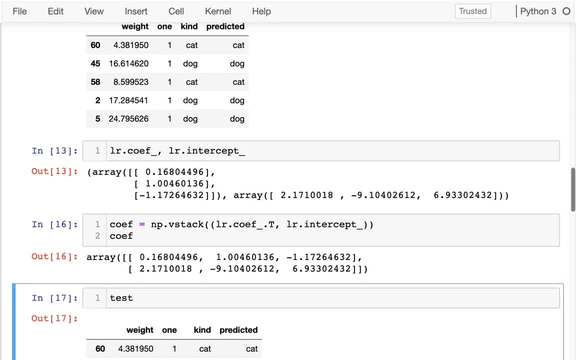 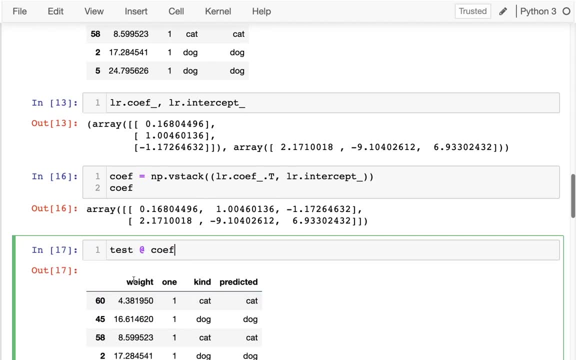 are right and so the way I can do that. well, if I just do this, this isn't going to work because the size isn't right. I only want to do it on on these first two columns. so let me take a slice of this. I think I want all the rows and only the first two columns, and- and this is kind of 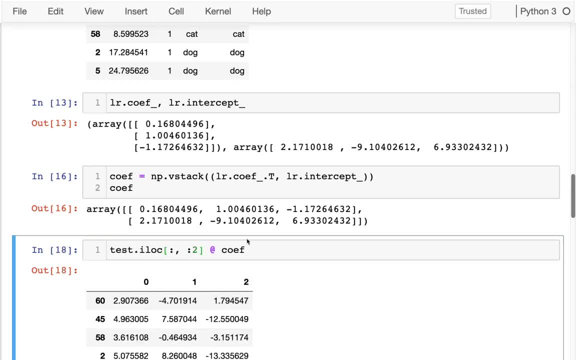 positional indexing. so I need to do that, and let me just be like, very clear here, let me actually get rid of this. this is a good refresher, okay, so there's my values. right, this is my data. and, and if I multiply it by by the first column, right, well, what is this one? let me just show you what this one is. 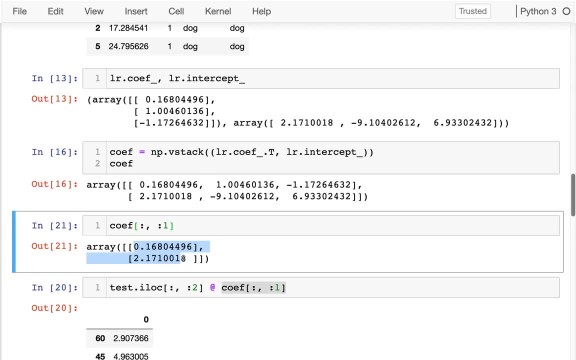 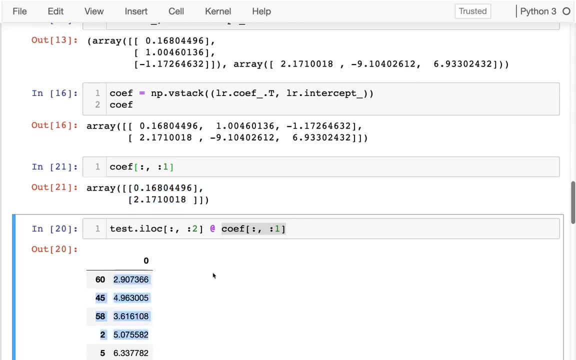 right, this is those first coefficients, right? if I multiply these first coefficients, which I'm imagining, or maybe for a dog, I get all of these scores here, right? And if I take the first two classes, the coefficient for both of those and I do the dot product of my 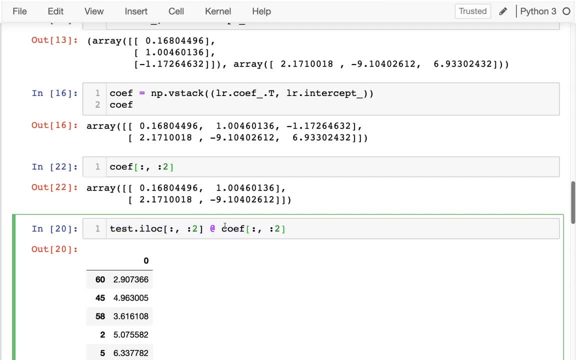 data times, both of these. adding another column to the second matrix just adds a second column down here, right, It didn't change my first one, right? And then if I add, you know if I want to get all the data right, if I want to get the third one, 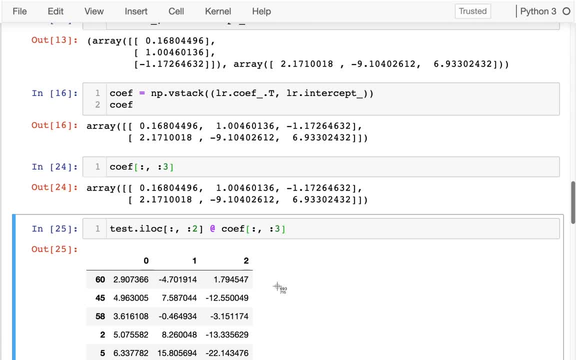 right, then it's just going to add another column down here without changing the other ones, right? So kind of, for each column I get in these coefficients, I get another column of output when I do my multiplication, And really at this point I don't have to do slicing because I'm just grabbing the whole thing. Okay, so I 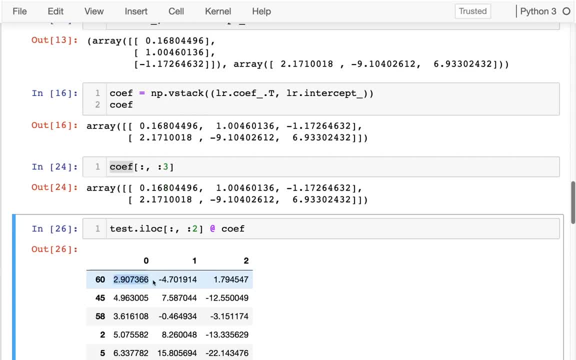 have this data, and what these things are is they're scores for how a dog's like or cat like each of my original rows were, And so, to really see this, well, what I should do is I should, I should let me get this in a data frame I need. 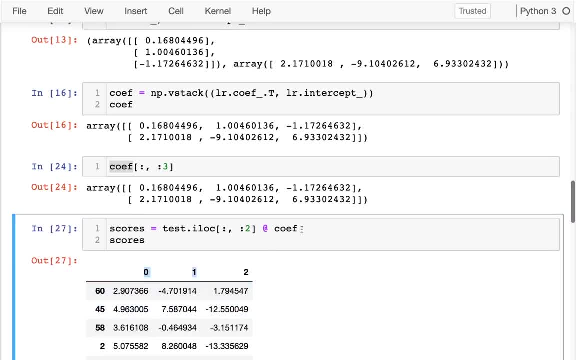 to have some names on here, right? I don't know which of these is dog, which of these is cat, and where do I have that? Well, I have it in my logistic regression, right, If I look at classes here. 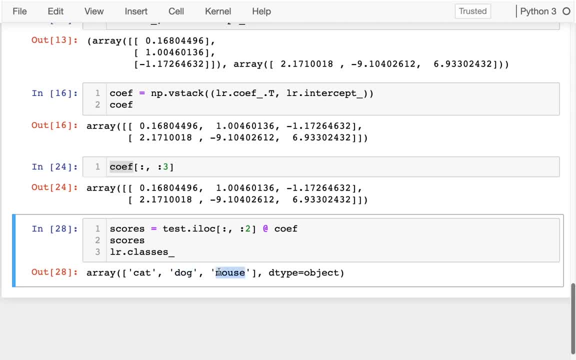 right, that'll tell me. it's, I guess, actually cat, dog, mouse. in this case, it ended up being alphabetical order, And so so what I can do is I can create a new data frame from this, and actually, you know, I don't want to. 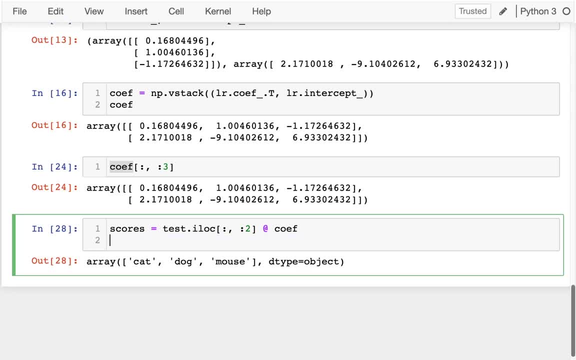 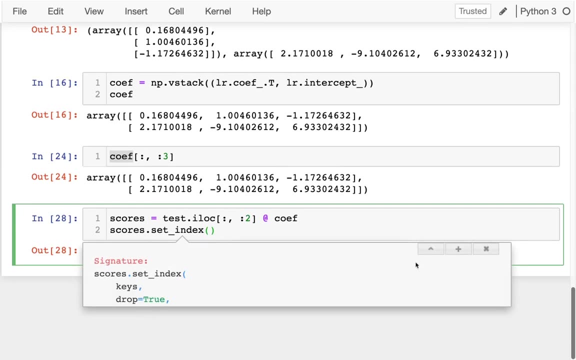 quite do that, but the best way to do this actually is scoressetIndex. I think it is. Let me show you how to have this in my notes. Great, This is going to let me kind of set the names in the index and replace existing columns. 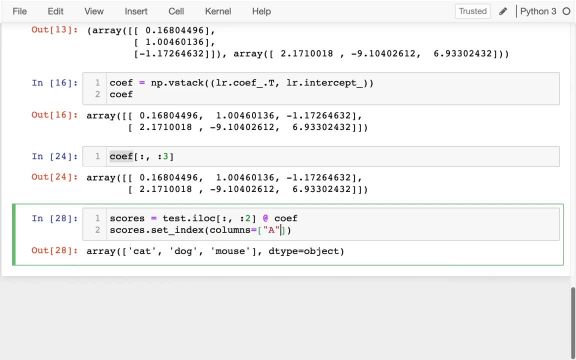 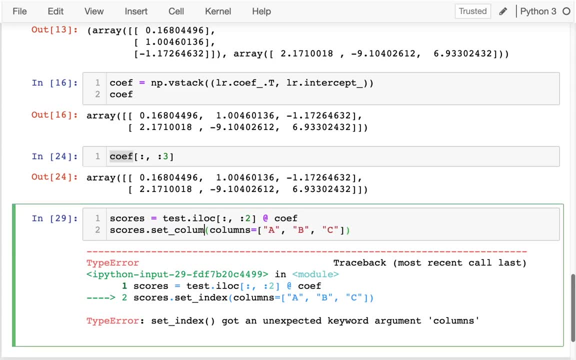 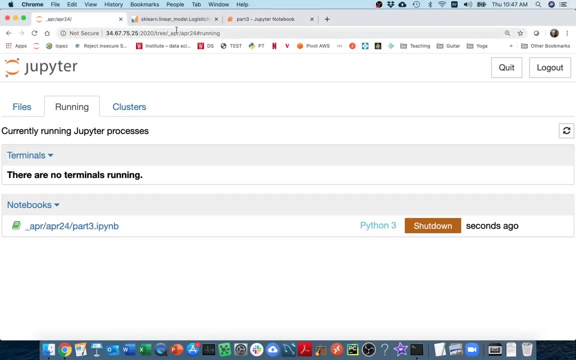 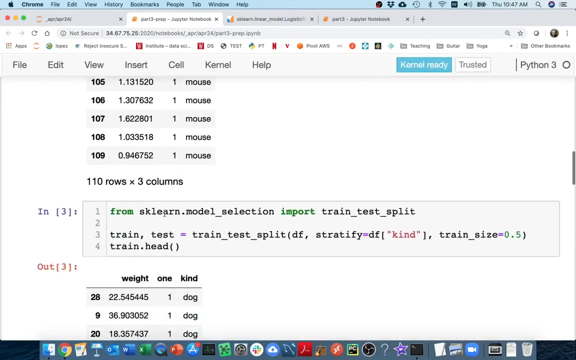 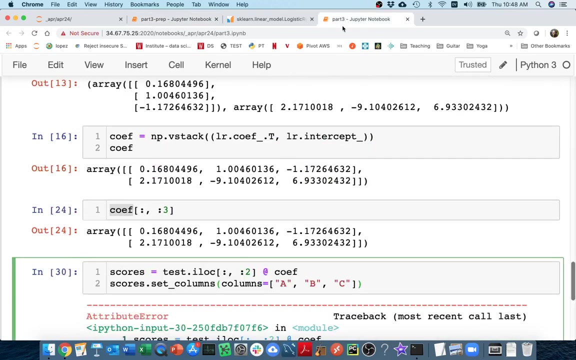 right. So when I say columns equals, you know A, B, C. What did I use before? Let me just check my notes here really quick. I'm apologizing for forgetting this. Okay, So so I'm going to call this first F. I'm going to call this first A. 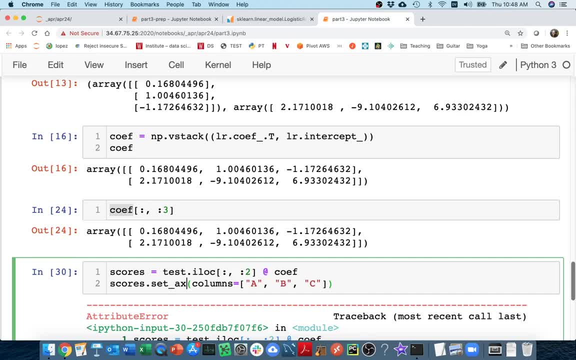 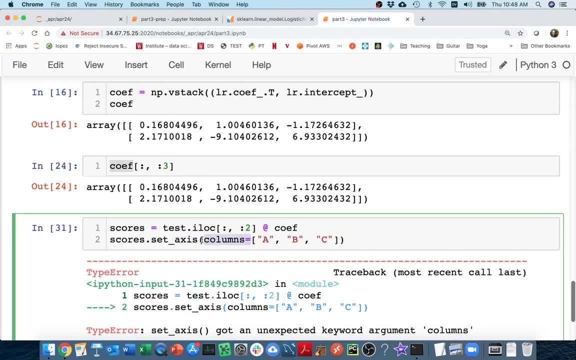 and then from here, let me, let me name it. What's down here? how do I rename columns? I have to say, you know, if I did that, I'd be setting the labels in the index right, the vertical. 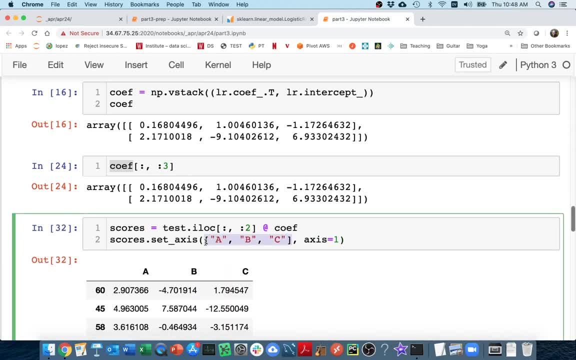 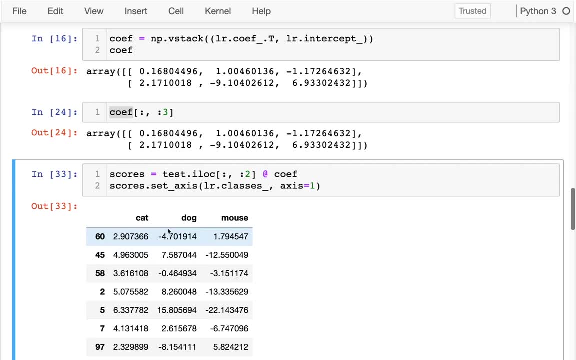 but one is horizontal. so I'm going to do that And then what I really want. sorry for the confusion there. I want to go back and use the classes from my logistic regression, right? So I'm kind of getting these three scores here and 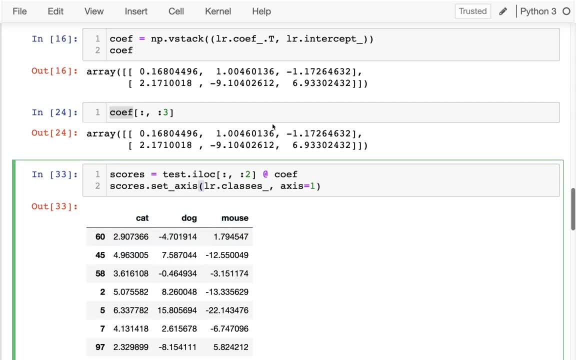 what else should I do? Well, let me just make it very clear. I'm going to directly putting those, I'm going to give it a better name. so for C and classes, I'm going to say C plus 4, just like that, so I can get a score. 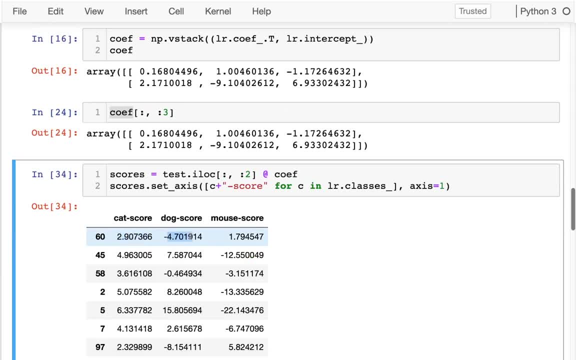 for each of them, and I'd really like this to just be between 0 and 1, so when I come back here, instead of I could use this right, I mean bigger still means it's more likely to be that class. so I'm just going to take 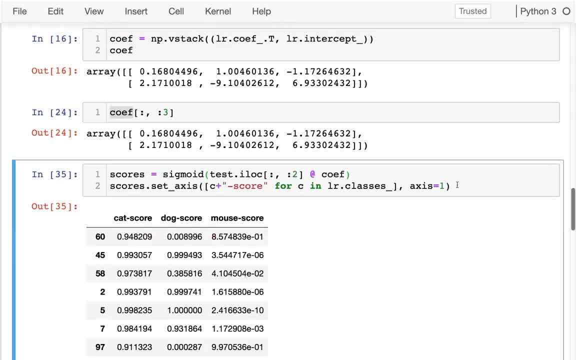 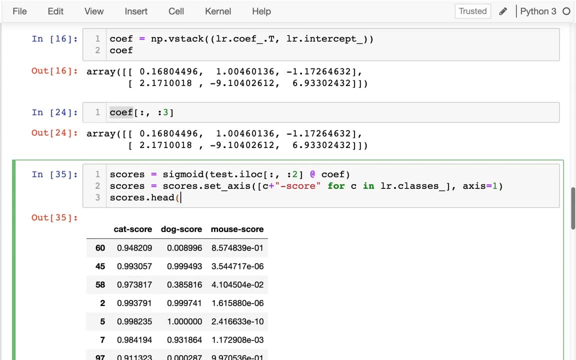 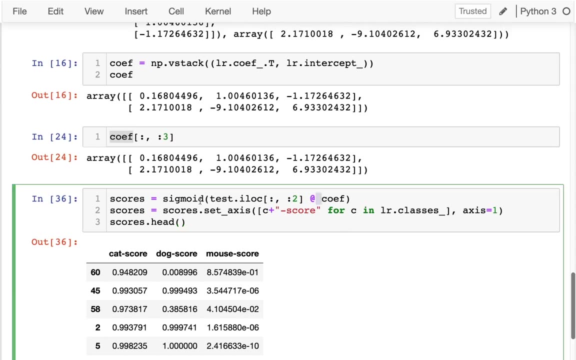 the sigmoid of this, to make them all nice numbers between 0 and 1, and I have these nice scores now, Right and just head, Okay. so what I want to do now is to combine this information right. I was using these coefficients on the 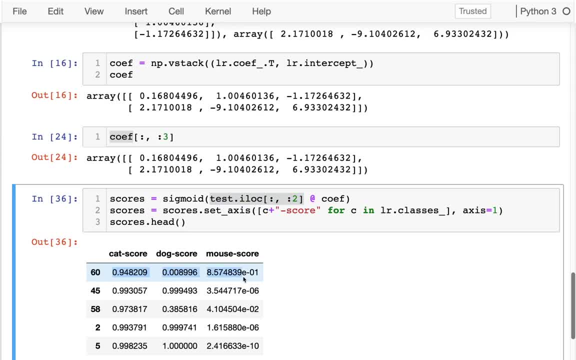 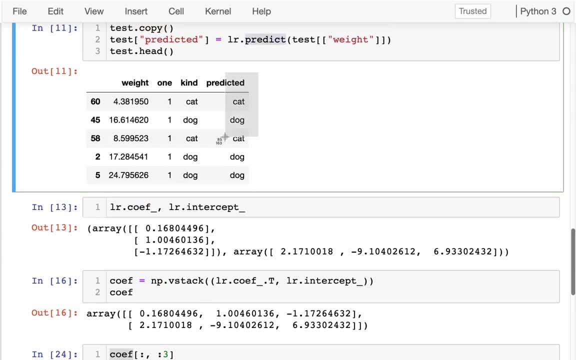 data to get, for each row, a score for cat, dog and mouse. and I'd like to go back and I'd like to show how that relates to what the logistic regression was predicting, right? So I'm actually going to take this test data and concatenate it with 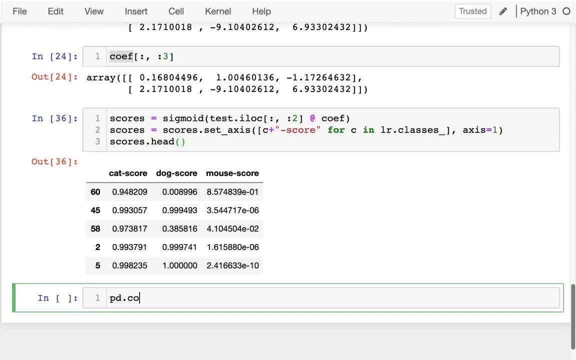 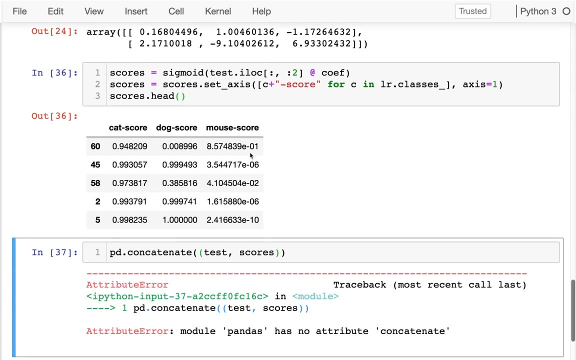 this scores data, and so I'm going to say pd, dot, concatenate, and when I do a concatenate I have to pass in two things. right, I have to pass in my multiple data frames in a tuple, and so I'm going to say test scores, and that's not how. 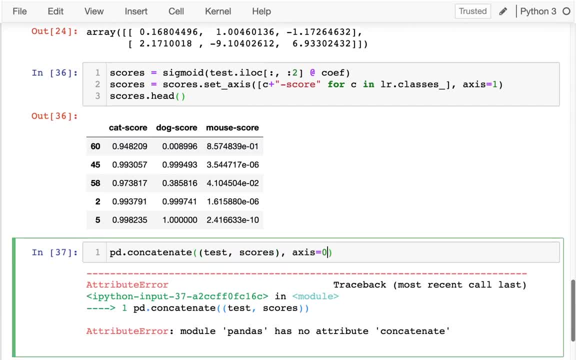 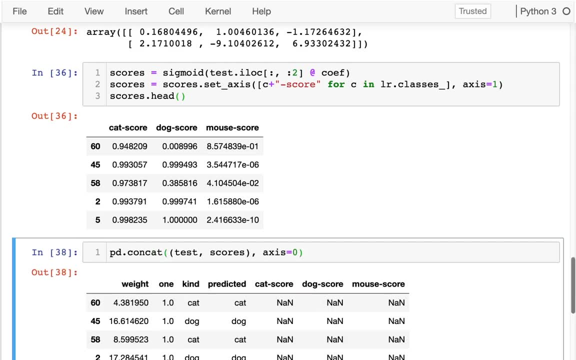 DreadBee is right now. the default is axis equals-. am I misspelling concatenate? Maybe it's concat, sorry. in NumPy it's that, and I don't. I don't think I'll ever see the results. so here we go. 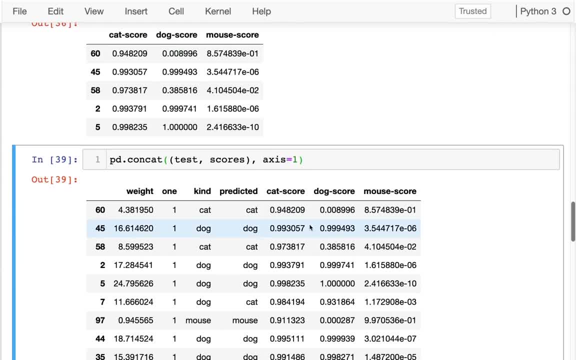 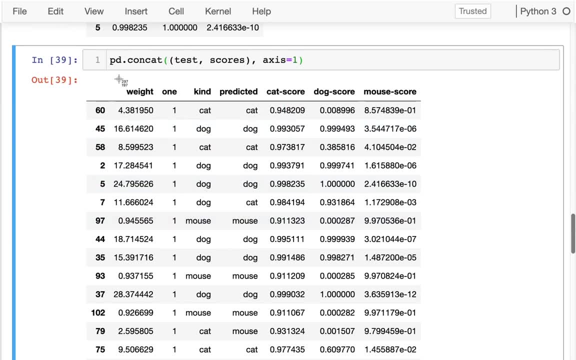 I don't want that. I want it to really be a cross right. So I'm going to do it like that. And then here, what I can see is: well, this is my original data. This one is what it actually is. 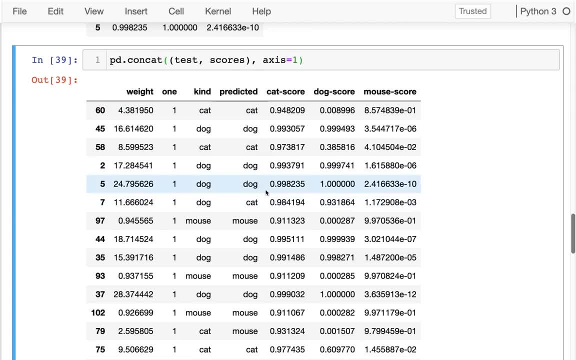 This one is what it was predicted to be, And that prediction was based on these scores right, all between 0 and 1.. I can see, for this first one, this 4-pound animal, the cat. logistic regression says 94%. definitely not a dog, maybe a mouse right. 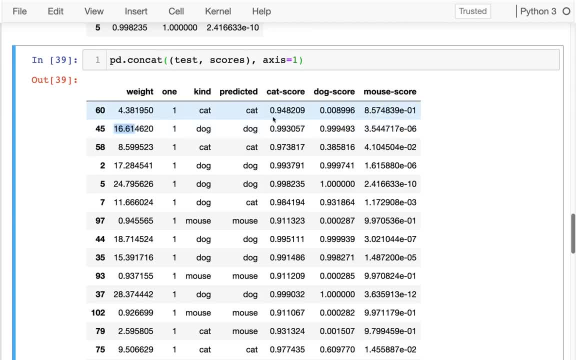 What about this one? Well, this one was kind of close. a 16-pound animal actually did pretty well on the cat score and slightly better on the dog score. And you may notice something here. is that, these numbers? right that? I'm showing you here the sigmoid of what we get when we multiply the coefficients by the data. 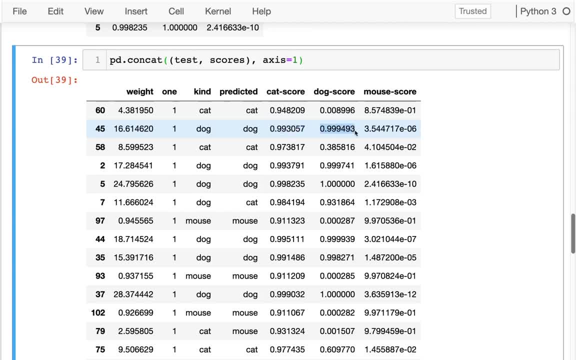 is often interpreted as a probability, but there's no guarantee those things are going to add up to 1, right, because these are kind of independently built right. So this one, what is this one? That one's a cat, I wonder. is there a mouse, right? 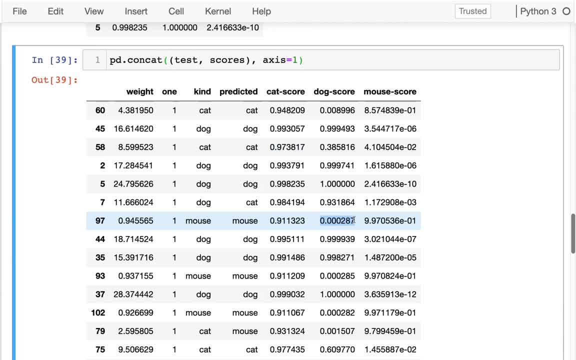 So for the mouse, I see I have 0.91, really small number, definitely not a dog- And this one, well, is 99.7, right. This one is kind of a little confusing. The mouse column is in scientific notation, right. 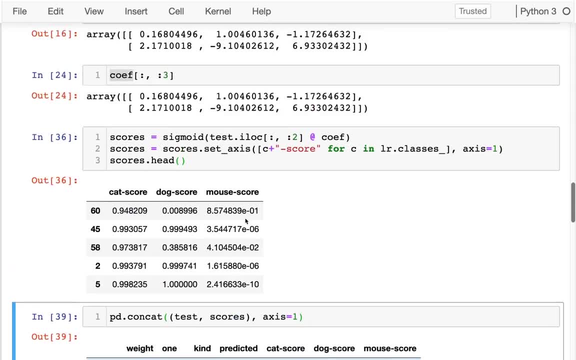 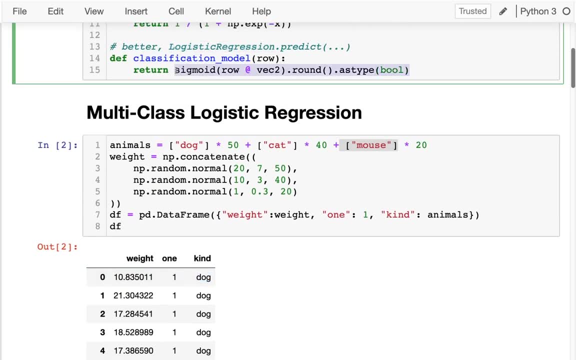 So that one was predicted to be a mouse. So that's all it's doing, Right? The hack here is that when we have multiple classes- right, we've already knew how to do binary classification- false or true- And if we have multiple classes, well, we just do this multiple times, one for each class, and then we kind of look at the score and see which one is doing the best.